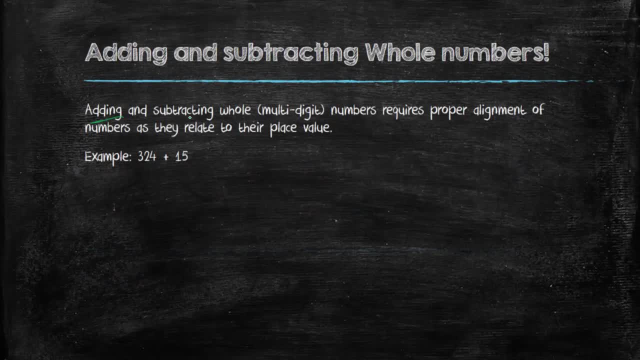 The first thing that we want to know when we're adding or subtracting whole numbers, especially multi-digit numbers, is that we require proper alignment of the numbers as they relate to their place value. So if you recall, place values is this table that we did earlier. And if you haven't seen it yet, please go see it. And this is a really quick version of it, but essentially the ones are here, the tens are here, the hundreds are here, the thousands are here, this is the ten thousands, and so on. And you could expand this table, this would be the hundred thousands. So if you had a number like, I don't know, 236,712, the two would be the ones, the one would be the tens, because there's one ten, there's seven hundreds here, so the seven here, the six here, the three here, sorry, and the two here. So why do we need to know this? Because when we come up to a number like this, 324 plus 15, we have to align them to the correct values in order for us to add correctly. So if we were to write it like this, 224 plus 15, right? This is 324, this is 15. 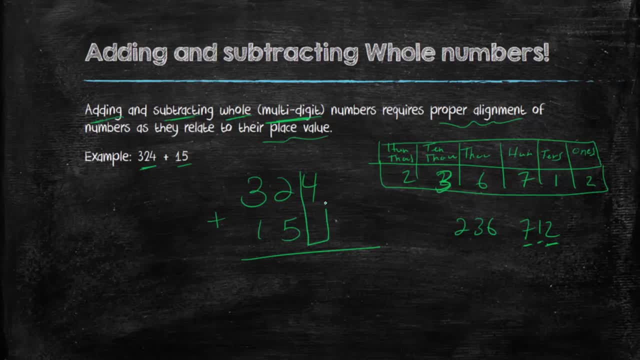 And if we add, we'll say, okay, we'll add this column, 4 plus nothing is 4, 2 plus 5 is 7, and 3 plus 1 is 4. So our answer is 474. Well, this is incorrect. This is fully incorrect. And the reason is right here. We misaligned the number. The 15, the 5 should be in the ones column, which is here. And the ones, should be in the tens column. So we actually moved everything to the side. So to appropriately write this, it'll be 324, let's just draw a line here, separate it, plus 15. The 1 is in the tens column, and the 5 is in the ones column. And the 1 is in the tens column. So we would add this, 4 plus 5 is 9, 2 plus 1 is 3, and 3 plus, well, there's nothing here. 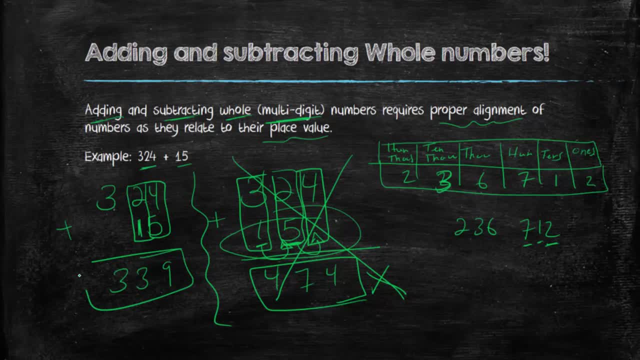 It's 3. So the correct answer is 339. Okay, so that's the hardest part. After you figure that out, it's really easy from here. So let's check this out. Okay, let's do these questions together, 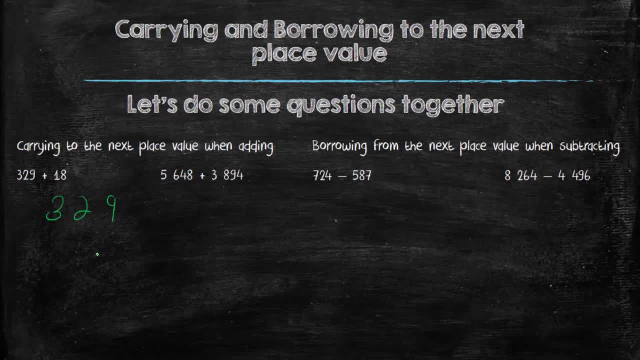 okay? 329 plus 18. Well, where does the 18 go? This is the ones, and this is the tens. So 8 and 1. And then we add 9 plus 8 is 17. So we put a 7 here. 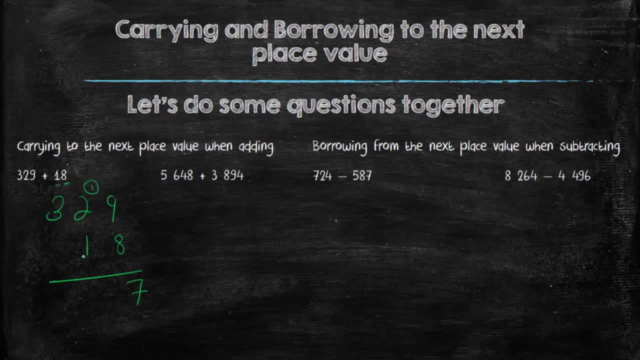 And we carry the 1 over here. 1 plus 2 is 3. 3 plus 1 is 4. And 3 comes down. There's nothing underneath. So the answer is 347. Let's do this one. 648 plus 3,894. The 4 is in the ones column. 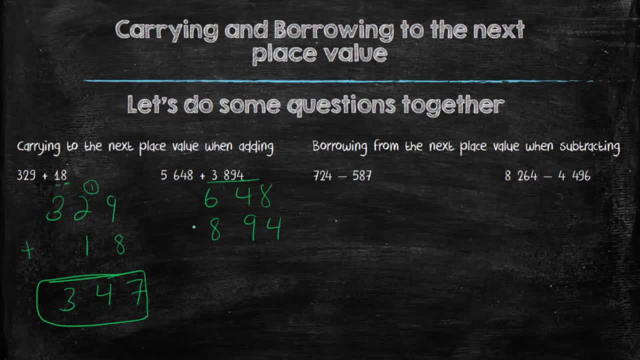 The 9 is in the tens. The 8 is in the hundreds. The 3 is in the thousands. Now there's no, there's nothing here. You could put a 0 here, but it doesn't make a difference. There's just nothing here. So let's go ahead and add this. 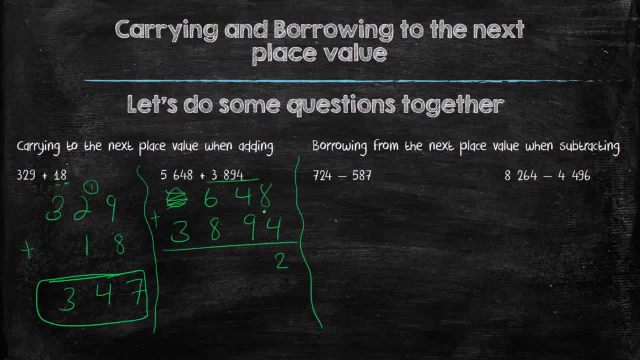 Let's just put some dividers here. 8 plus 4 is 12. So we put the 2 here, and we carry the 1. 1 plus 4 is 5. 5 plus 9 is 14. Put the 4 here. We carry the 1. 1 plus 6 is 7. 7 plus 8 is 15. 5, and we carry the 1 here. 1 plus nothing is 1. 1 plus 3 is 4. So the answer is 4,000. 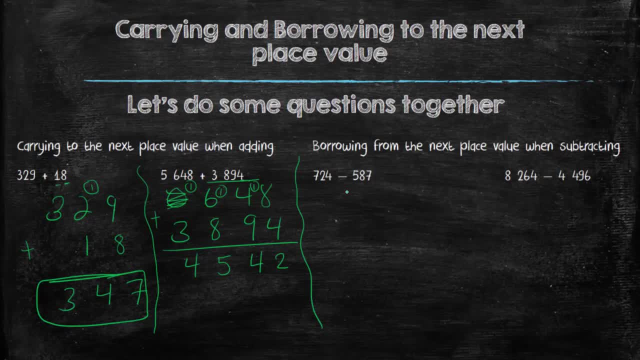 554. Let's do some subtraction here. 724 minus 587. 4 minus 7. Well, we can't do that. So we have to borrow from here. So this becomes a 1, and because we borrowed 1 ten, this becomes a 14. Correct? So 14 minus 7 is 7. 1 minus 8 is 14. we can't do that so we have to borrow from here so this becomes a 6 and this becomes an 11 11 minus 8 is 3 6 minus 5 is 1 the answer is 137 and this is also